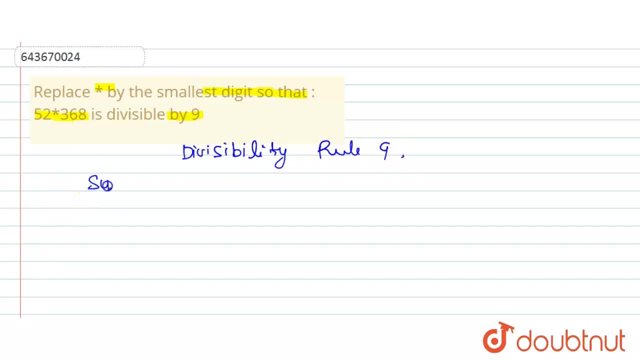 So if a number, that is, that means sum of digits, sum of digits of a number will should be divisible by 9.. Okay, then the given number will be Complete. given number will be divisible by 9.. Okay, So here the number which is given as 5 to. 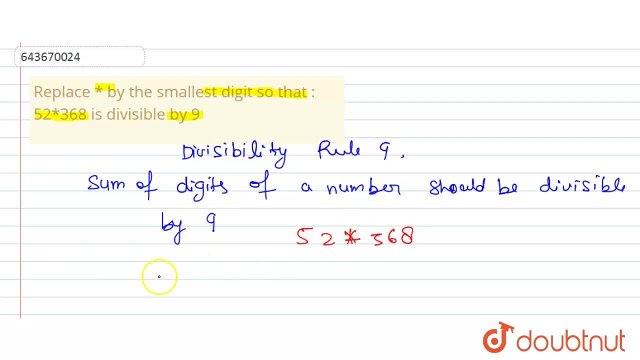 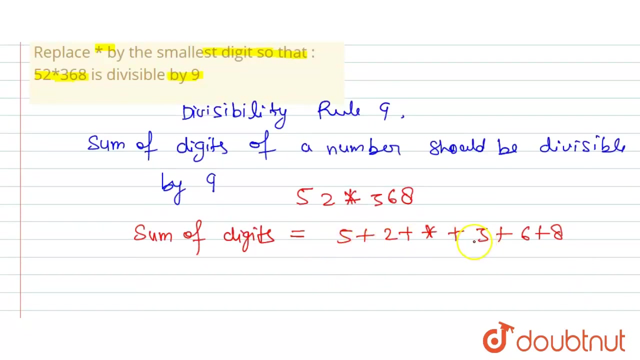 star, 3, 6, 8. so sum of digits Here. if we talking about the sum of digits, so this is going to be equal to 5 plus 2 plus star And plus 3 plus 6 plus 8. Okay, so 5 plus 2, 7 and plus 3, that is 10 and plus 6, 16 and 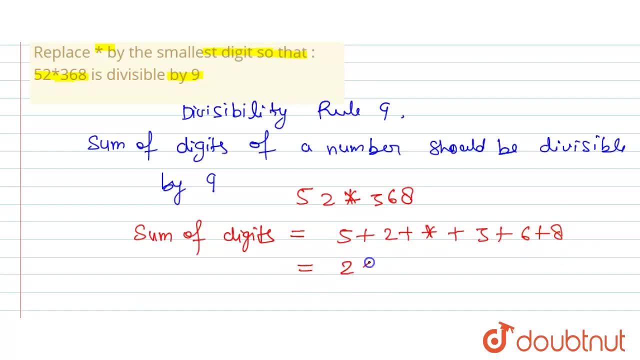 plus that is 8.. So this is going to be equal to 24 And plus star. So, my dear student condition is that the sum of digits should be divisible by 9. Okay, so this is the number which is 24. now star, the smallest number. what is the smallest number which is replaced by a? 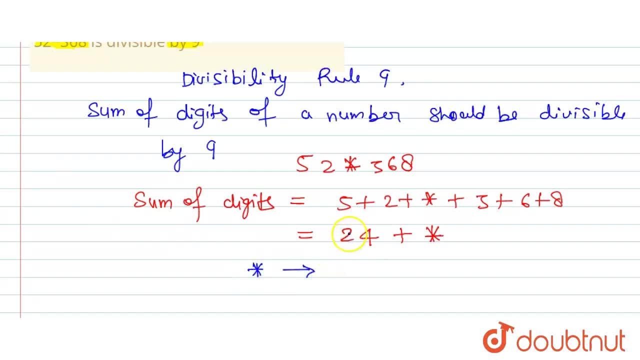 star. so here we will find the 20. what will should be added in the 24, then the. it become multiple of 9. so if either the smallest number here will be used, that is 24- sorry, 24 plus 3, so that is becomes equal to 24 plus 3, this is equal to 7. so 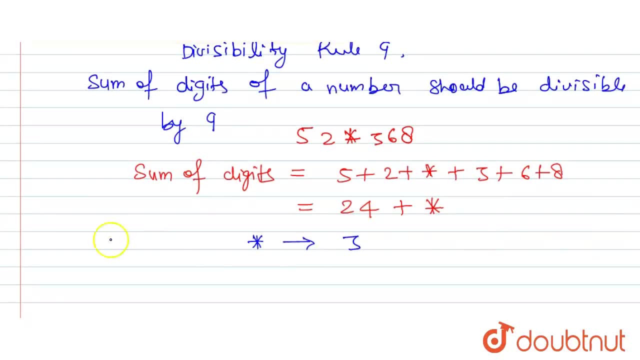 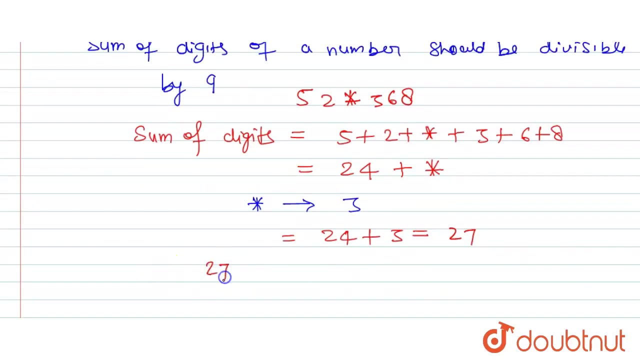 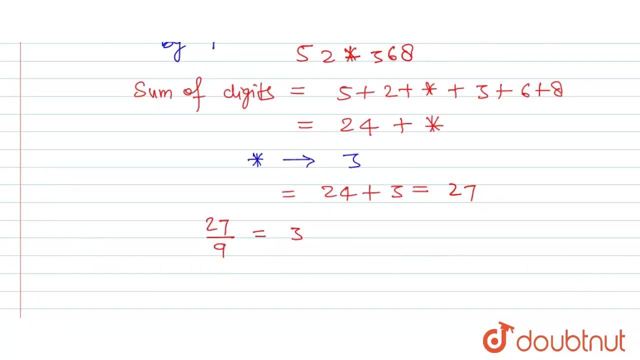 a star can be replaced by 3. okay, so if we will add here 3, so this becomes 24 plus 3, so this is gonna be equal to 27. okay, now check we will. 27 is divisible by 9, or not? so, yes, this is a multiple of 9, so star.